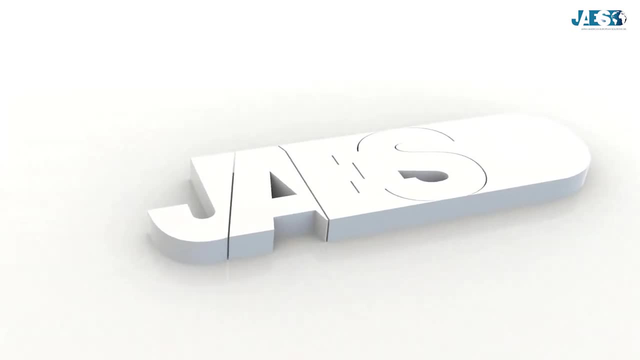 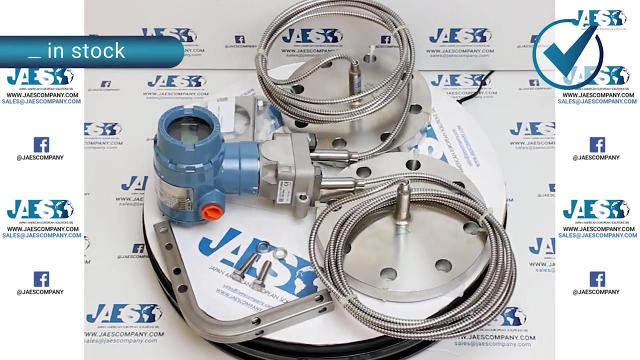 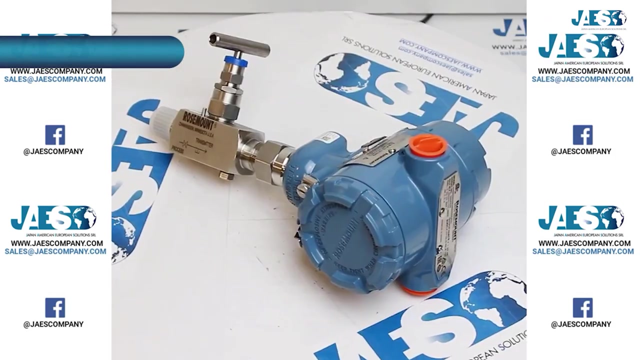 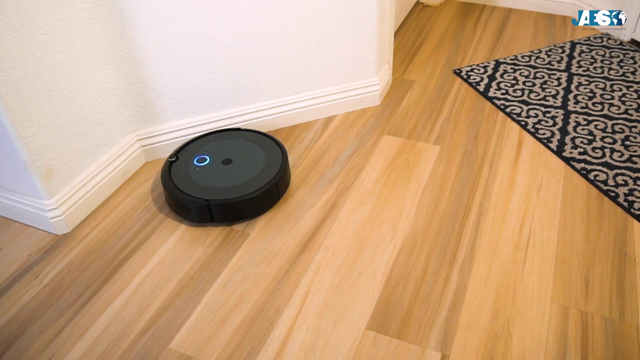 in any technological field. JAWS has been in the Industrial Supply business for over ten years and has become partner of some of the most important companies in the industrial automation market by supplying every type of sensor and transducer. Sensors and transducers are able to acquire information. 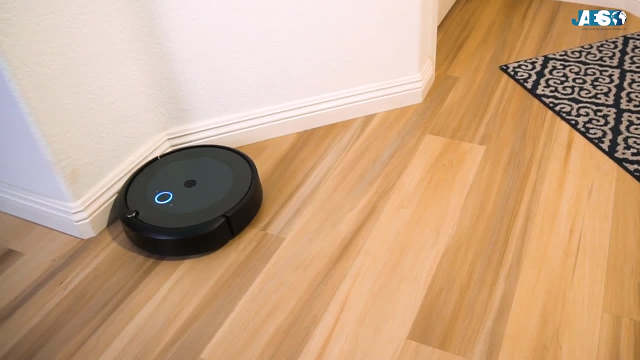 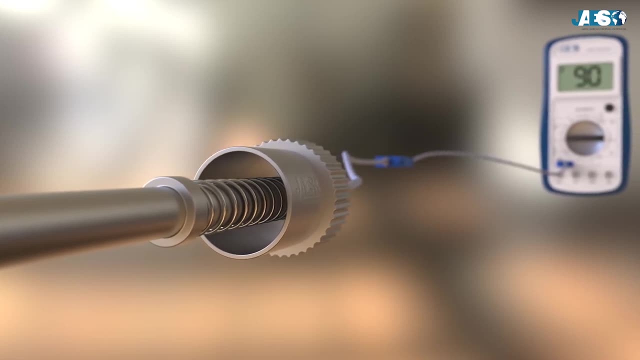 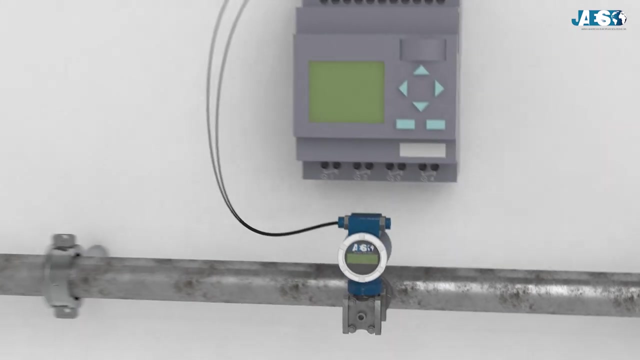 from the outside according to the type of physical quantity they measure. eg. A microphone is a sound sensor, a thermocouple is a temperature sensor, a photodiode is an optical sensor, a pressure meter is a pressure sensor and etc. Physical quantities are all the properties. 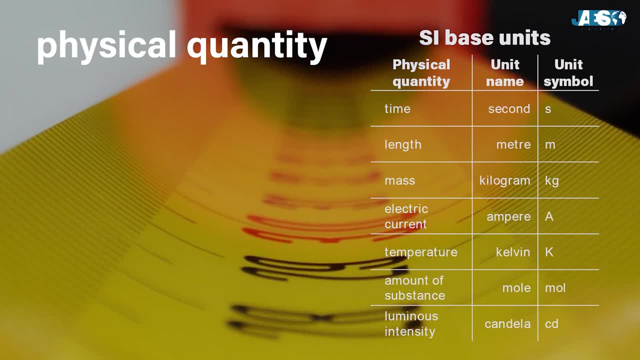 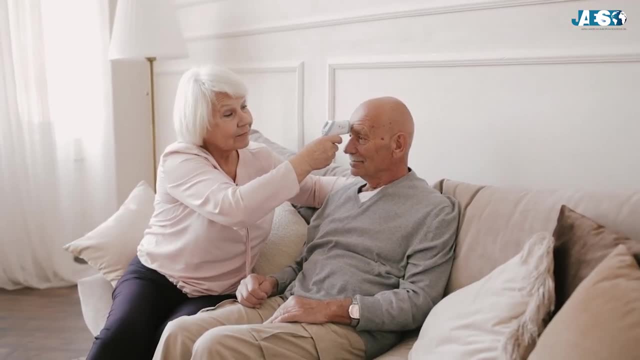 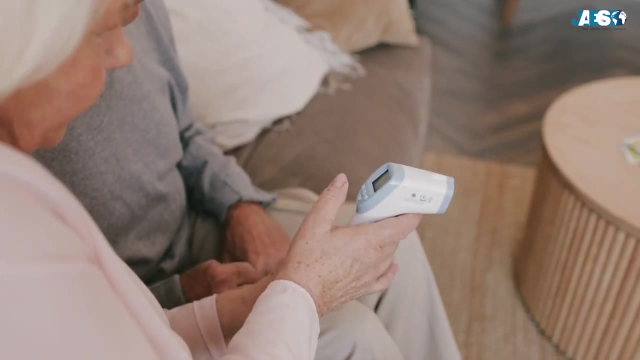 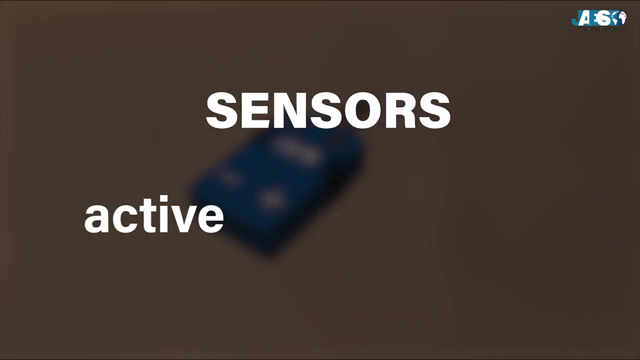 of a phenomenon, and so can be expressed quantitatively by a number. Sensors and transducers, after detecting the values of a physical quantity, transform its variations into electrical signals. So what is the difference between a sensor and a transducer? Sensors are divided into active or passive. 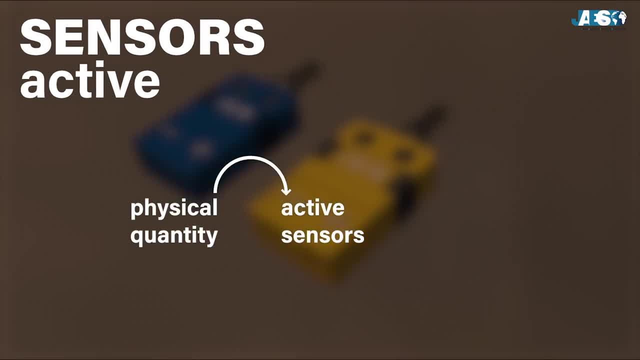 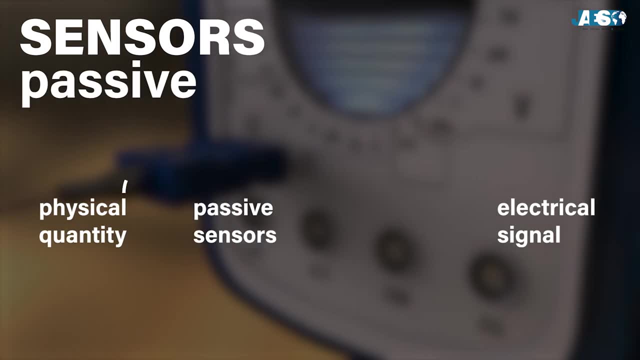 Active sensors are able to transform a physical quantity directly into an electrical signal, without needing an external power supply. Passive sensors, on the other hand, do not produce an electrical signal. A transducer is an electrical signal that can be used immediately. Instead, they must. 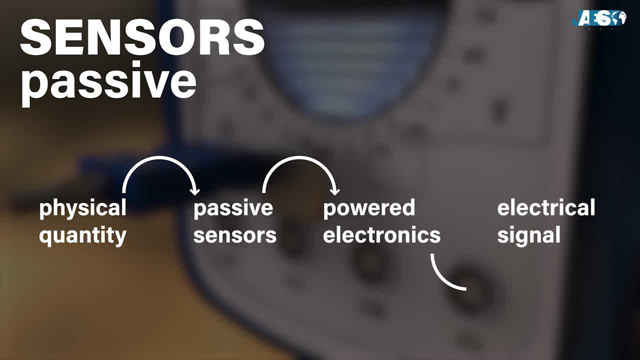 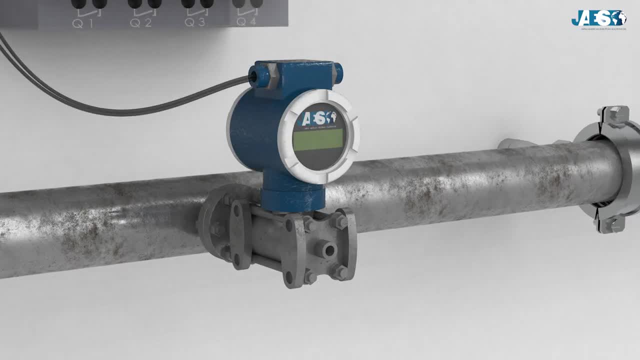 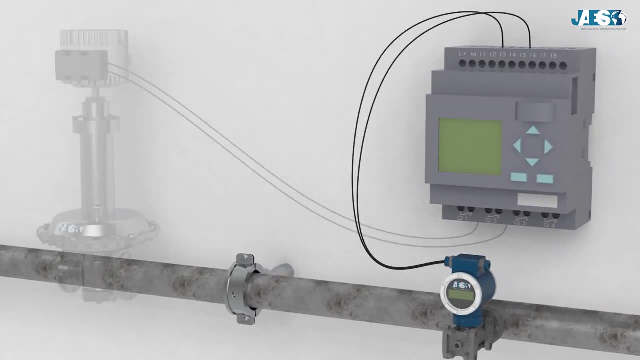 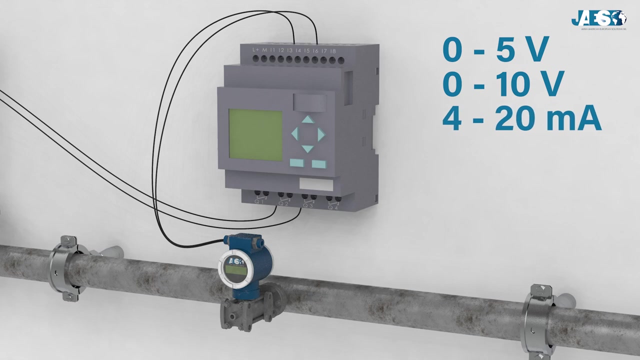 be accompanied by powered electronics that will produce the correct electrical signal. The union of these two components is the transducer. These signals are then transmitted to a controller, which reads and interprets them. Standard electrical signals are a range of electric tension, typically 0 to 5 volts or 0 to 10 volts, or electric current, usually 4 to. 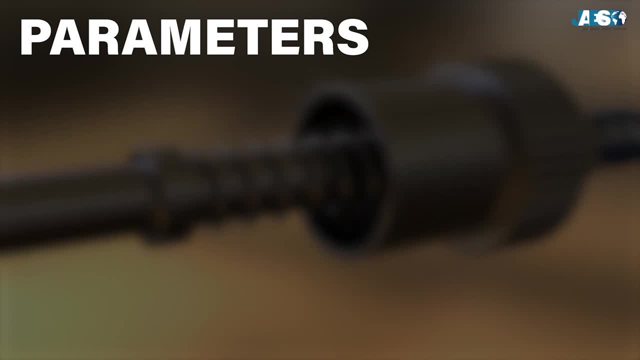 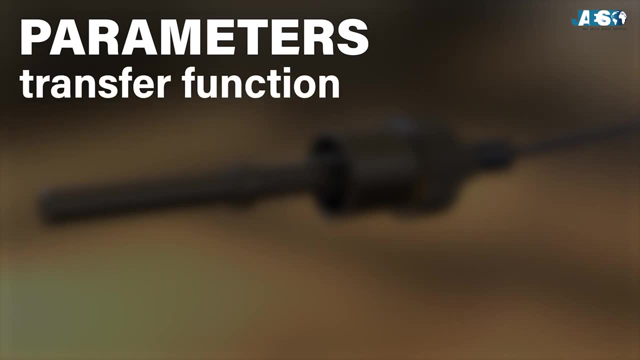 20 milliamps. What are the various parameters that sensors and transducers have? First of all is the one called transfer function. Sensors and transducers have an input signal and an output signal. The output signal varies as the input signal changes and is related. 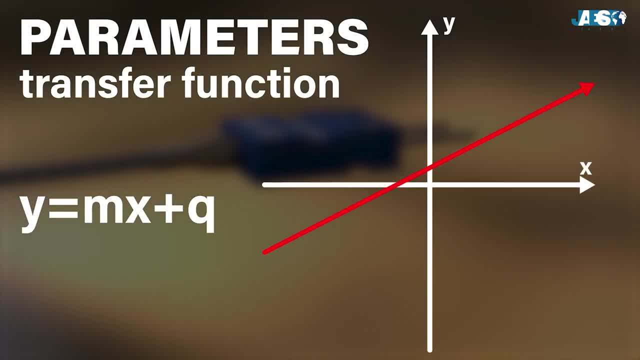 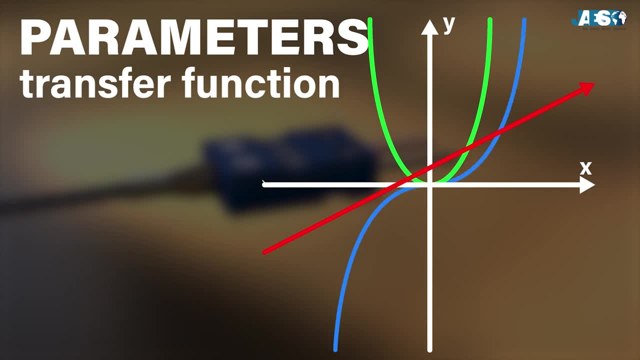 to it by a mathematical function called the transfer function. 2. Transfer function. 2. Transfer function. The transfer function can be linear, quadratic, cubic, exponential or logarithmic. The most commonly used transducers either have a linear transfer or are operated in the range where the transfer is more linear. 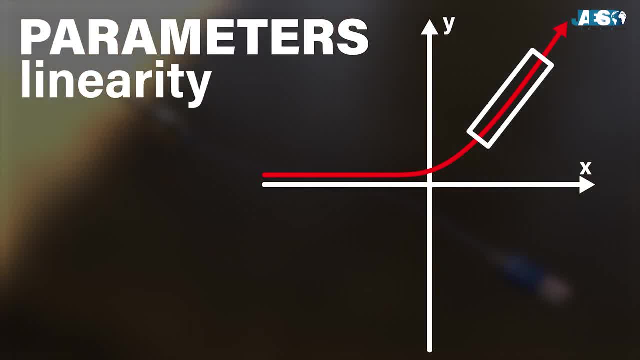 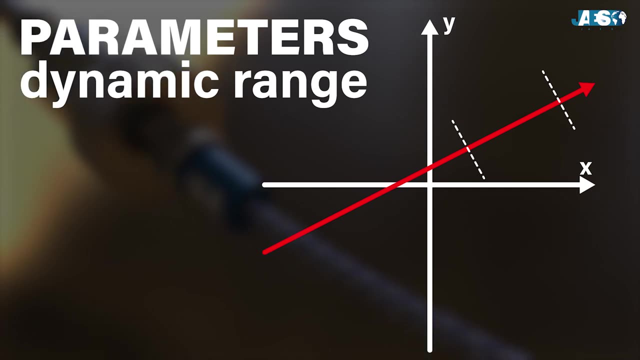 Linearity is, in fact, another important parameter that measures nonlinearity, error of the transfer function. Another primary parameter is the dynamic range, also known as the functioning range, which is the range of input values that the transducer or sensor can operate without damage. 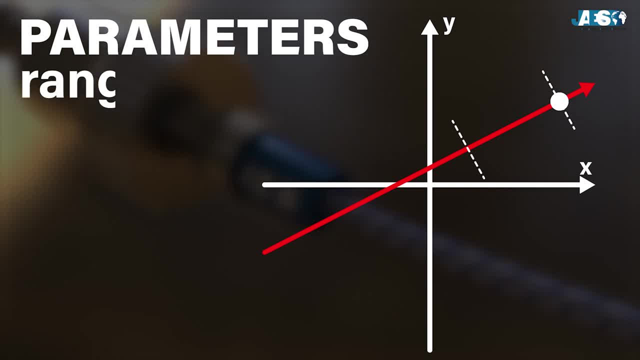 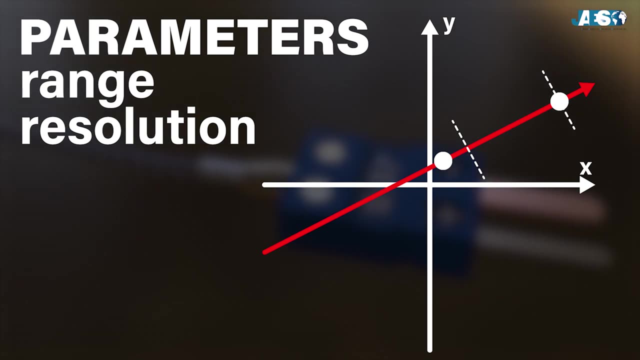 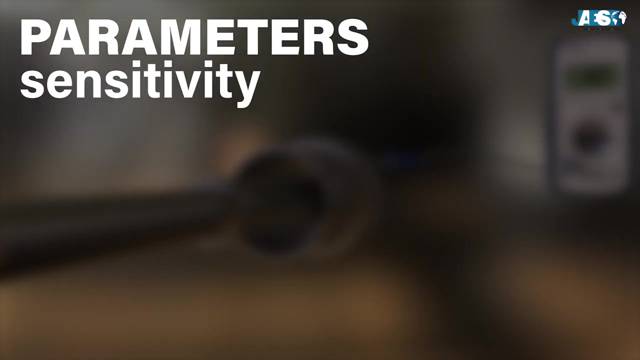 The maximum value of the dynamic range identifies the range of the transducer, whereas the minimum value designates the resolution. A good sensor or transducer has a low resolution ie. It can detect signals of a small value and a high range, so as to have a very large dynamic range. 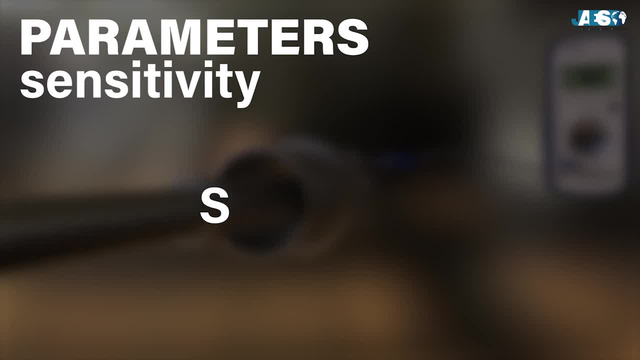 Another crucial property is sensitivity. The sensitivity of the transducer is the relation between the variation of the output magnitude and that of the input which determined it. The instrument will be very sensitive when, for the same variation in the input variable, the variation in the output is very high. 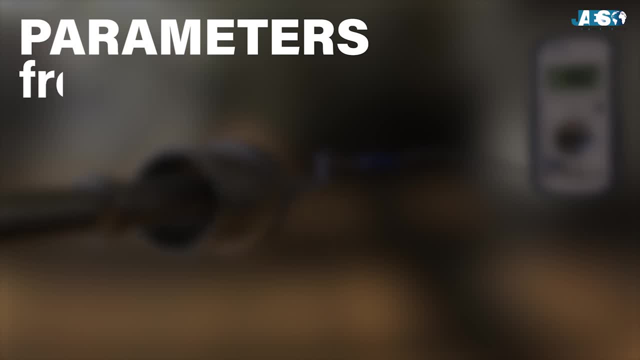 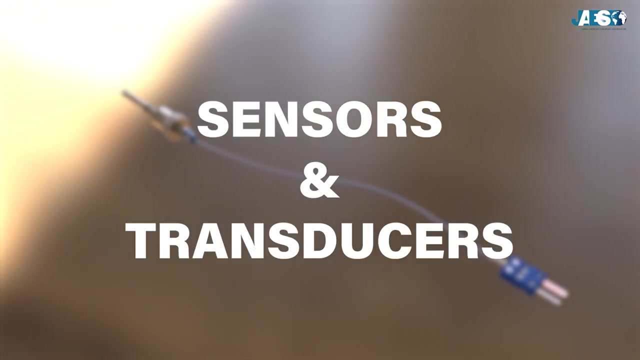 Frequency, on the other hand, is the time taken by the transducer to transform the variation of the input magnitude into the output signal. It is important to note that the smaller the size of the sensor, the faster its response tends to be. Let's see some practical examples to understand how they work. 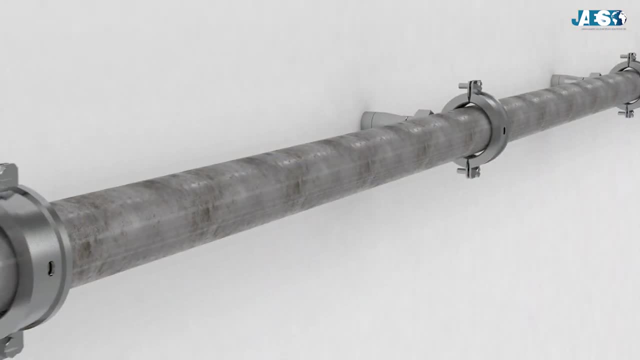 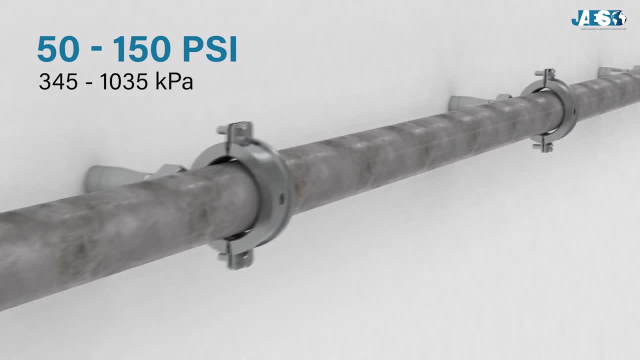 Let's say, for example, that we want to monitor the output. Let's see how this works. Let's say this works. Let's say a single keybalancer is not the only way to detect how classically the output is arranged. 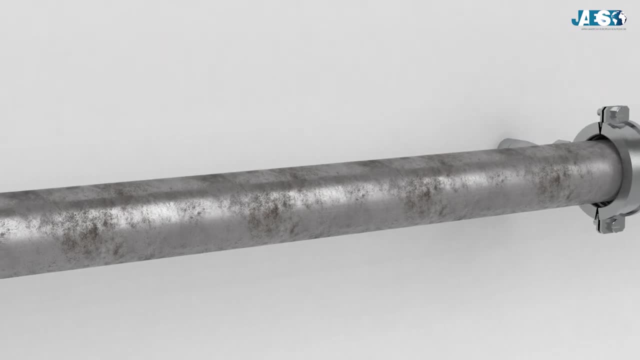 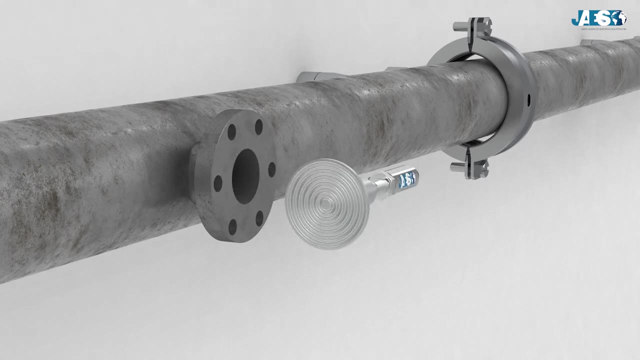 Cancellation of a single keybalancer can only be acted upon a single data which can be translated. In our practice ofâte, hardly any sub hommes of energy does theuri takimor. One device is not the only way to detect the output and precisely what pre- pantalla. 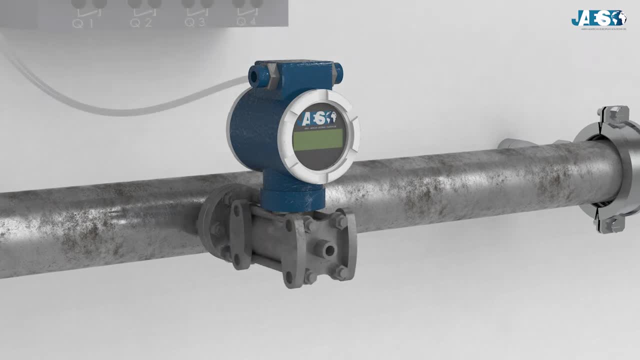 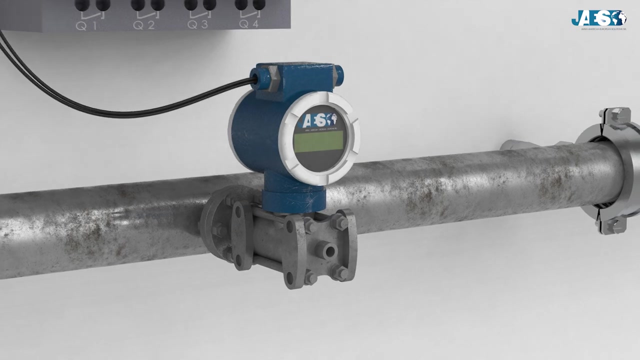 with which multidimensional signals are created over a interval of a certain number of odd hours, calibrated to the minimum and maximum pressure range, linearizes, compensates and expands the signal, which in this case is a range between 4 mA and 20 mA. The signal is sent to the 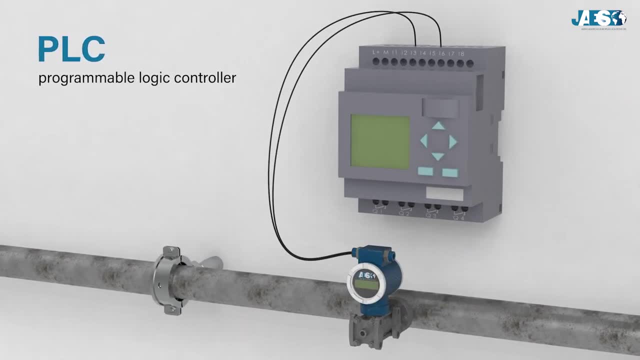 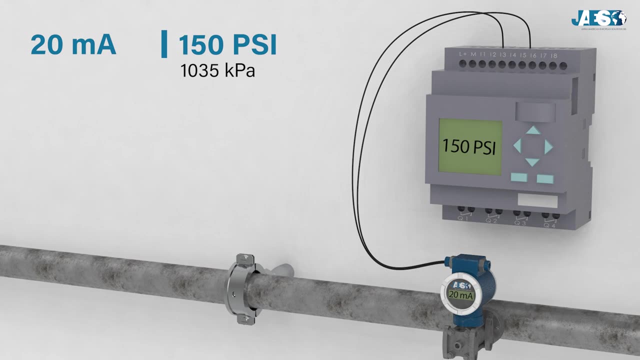 programmable logic controller, PLC, that is a computer that interprets the current at 20 mA in a pipe pressure of 100 psi or 1035 kPa, 4 mA in 50 psi or 345 kPa, and for example. 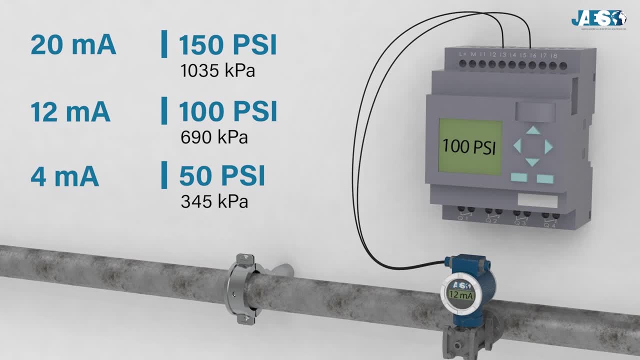 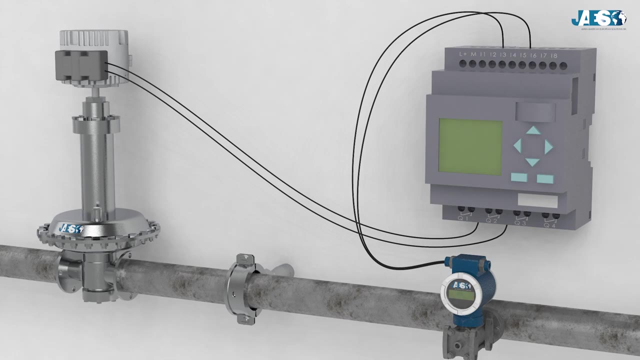 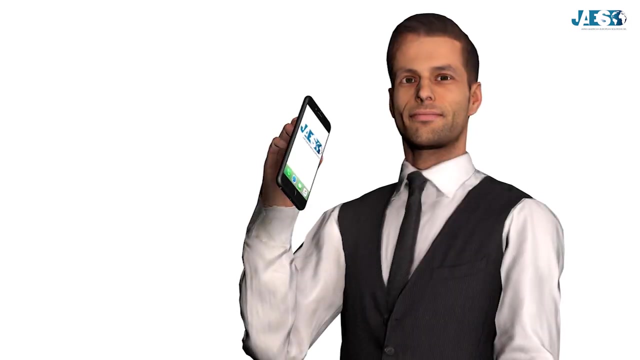 12 mA in 100 psi or 690 kPa- 50% of the pressure range. Now the controller can determine the pressure and, if necessary, it changes it by sending a signal to an actual controller. In our second example, we'll examine the main components of a smartphone during a phone call. 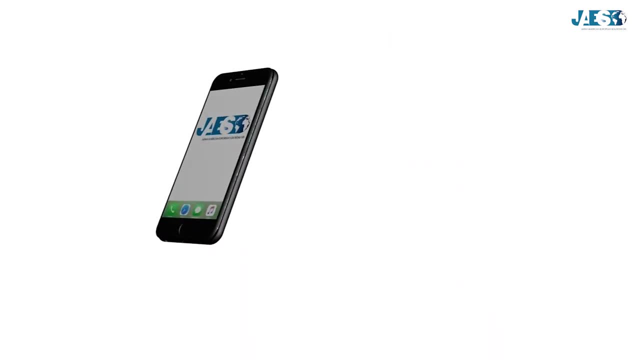 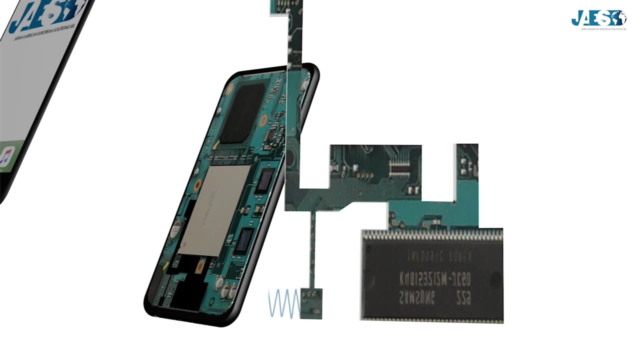 When we start a phone conversation, our voice is recorded by a microphone. The microphone is nothing but a transducer capable of converting sound pressure waves into electrical signals. Once the wave of our voice is converted into an electrical signal, it is received By a microelectrical mechanical system, MEMS, which interprets it into binary code. 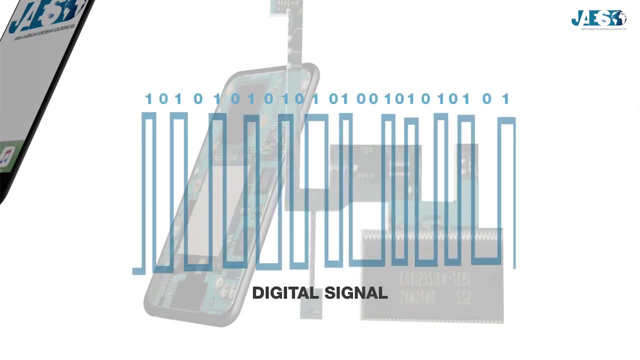 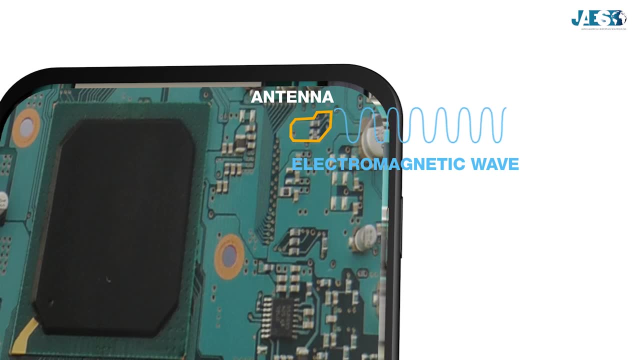 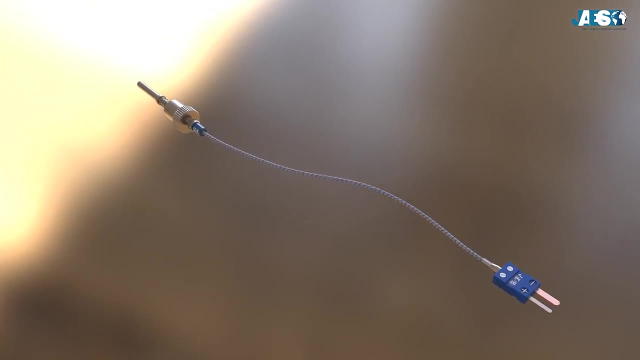 of many zeros and ones digitizing it. In this way our voice can be easily stored and eventually sent to an antenna. Another example is the thermocouple, a temperature transducer. It is a probe consisting of two wires made of different metals. 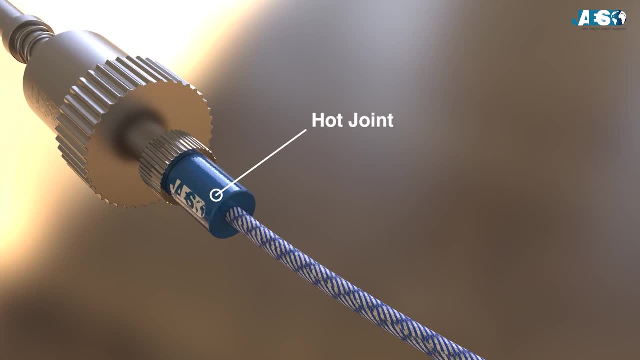 where one extremity is the temperature transducer and the other is the temperature transducer. The thermocouple is the temperature transducer, where one extremity, called the hot junction, is placed in the environment to be measured, while the other extremity, called the cold junction. 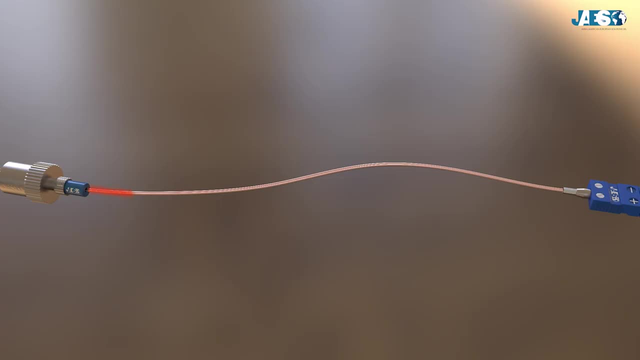 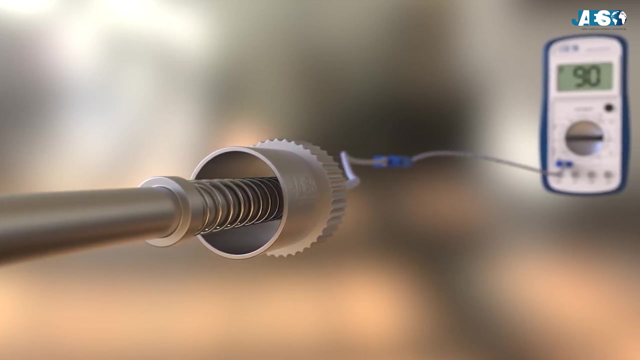 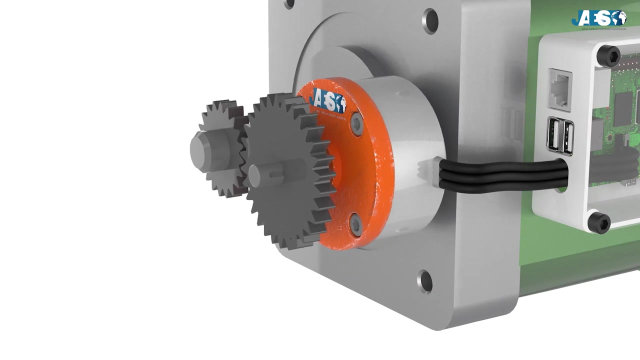 is connected to a measuring instrument. The heat difference between the two extremities generates a displacement of electrons in the cooler part, creating an electric potential difference with a specific voltage from which the measuring instrument can interpret the temperature. Let's now see an object called the rotary encoder. 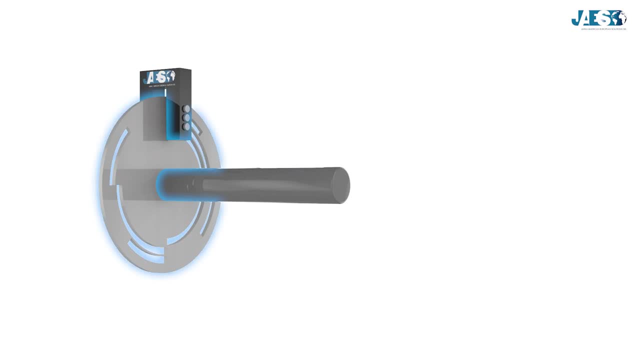 We can see on the inside, there is a slotted disc placed on the rotating shaft, used together with light sources and fixed photo sensors, usually photodiodes. As the shaft rotates, light sources illuminate the coating disc and the transmitted light that manages to pass through the grooves meets optical sensors, which allow the battery's. 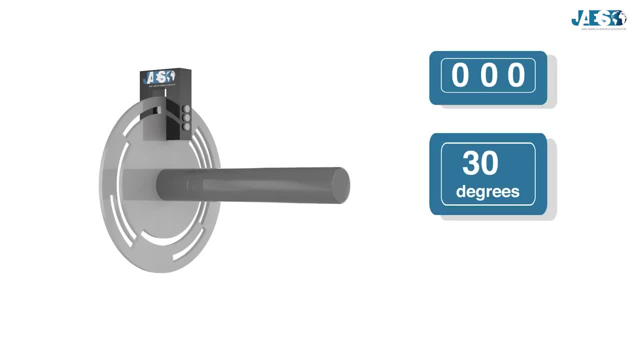 to be charged by the hot ohms. This way, we are able to take an audio cable out of a. meets optical sensors capable of producing, with output signals, a unique code pattern which determines the exact position of the shaft, A PLC is always required. 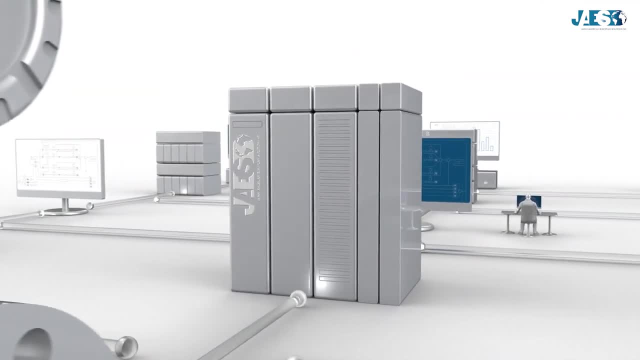 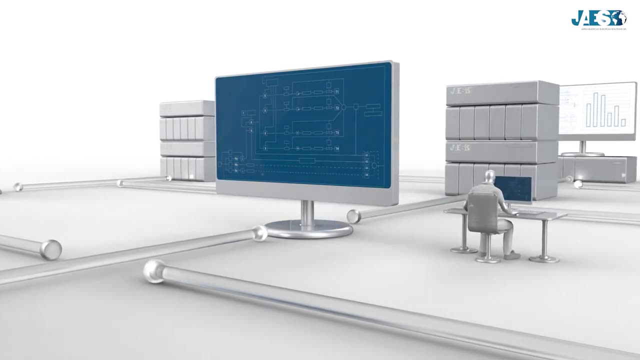 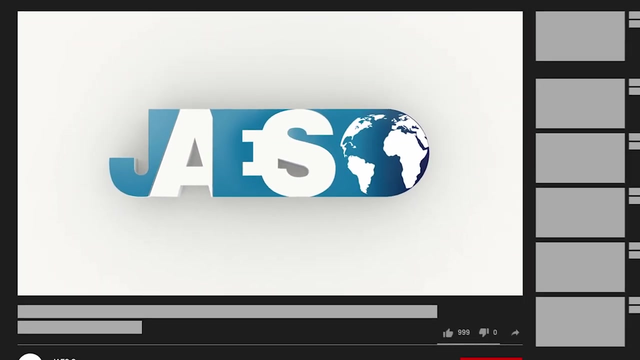 to interpret sensor and transducer signals. If you are interested in understanding how PLCs and DCS work, please watch our previous videos. If you found this video useful, please let us know by leaving a like and a comment. You can also share it. 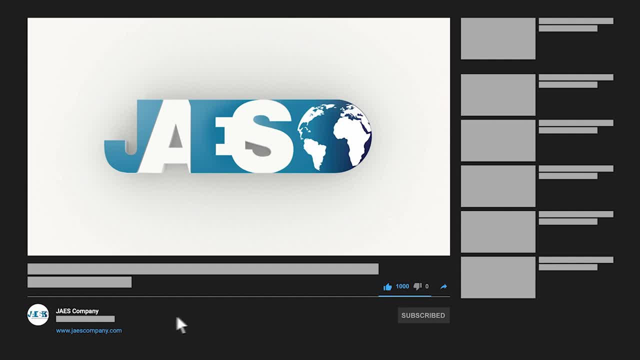 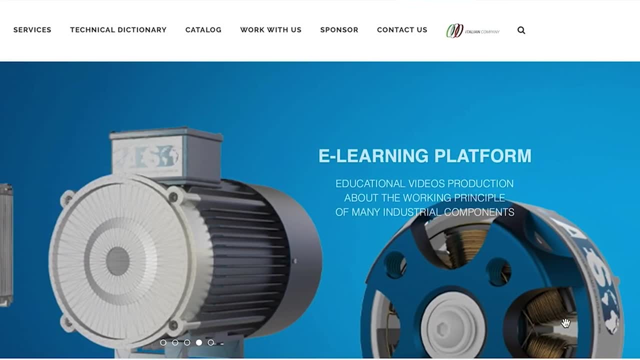 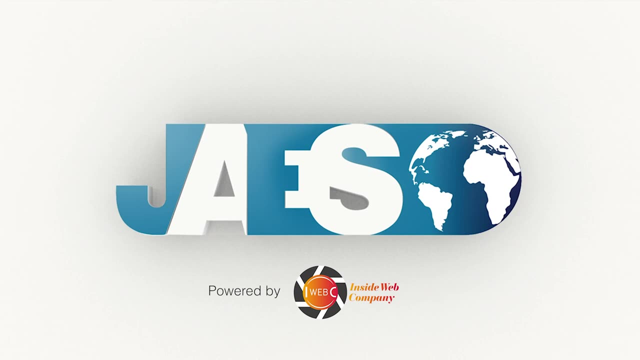 And don't forget to subscribe to our channel. Please visit our website, JawsCompanycom to find out our next projects. Thank you.